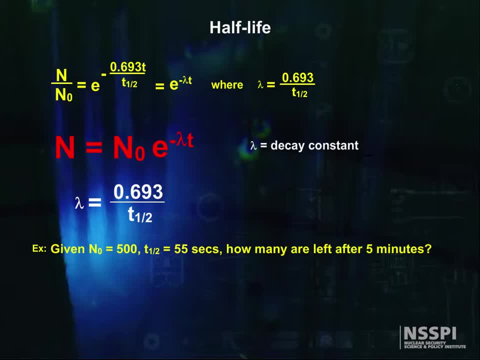 Get your pencil and paper and do it again. I get 11.41 atoms, And just between you and me, I think it's kind of hard to have 0.41 atoms. Well, what's wrong with our equation? Nothing is wrong with our equation. In fact, our equation is better than reality. What? 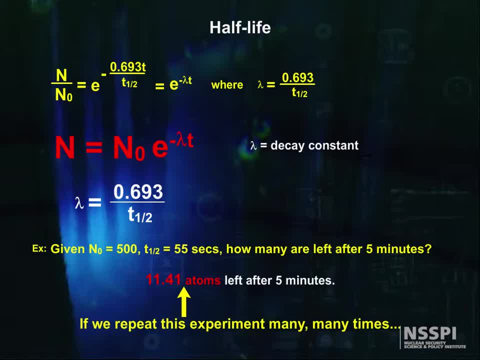 equation says is: if you repeat this experiment many, many times on average, you will have eleven point four one atoms left after five minutes. this is somewhat the same as the average couple and in the United States having two point one, three kids, or two point four two neutrons emitted during fission, the 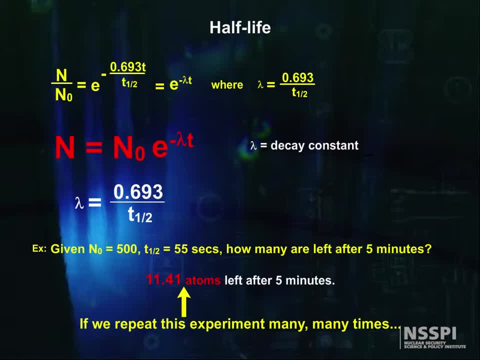 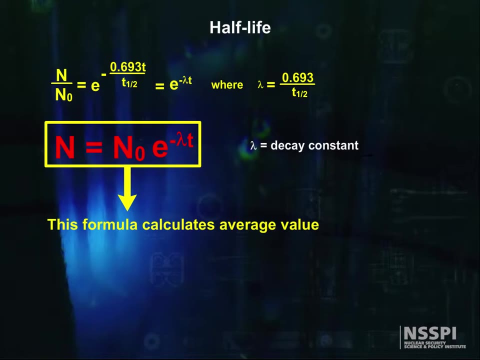 equation describes the expected value, to use the statistical term. there's another wrinkle, because it's statistical. our formula gives the average value in real life. if you have a small number of atoms, the odds that you will get exactly the answer given by the formula, even if it's a whole number, is small. well, how can? 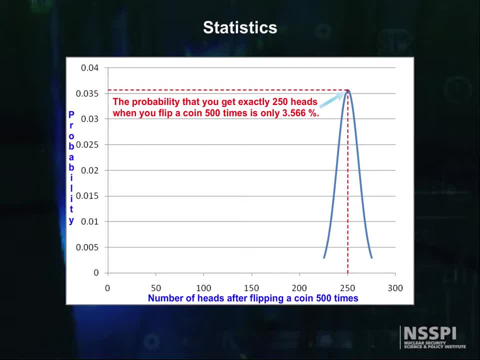 this be. let's think of flipping coins for a minute. if you flip a fair coin 500 times, how many heads do you expect? 250, right? the odds that you get exactly 250 heads when you flip a coin 500 times is only three point five six. 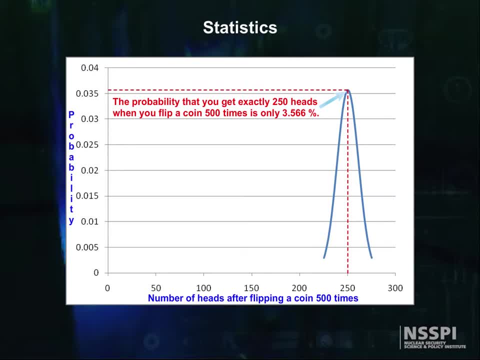 six percent. to be clear, if you repeated this experiment many times, your average number of heads will get closer and closer to 250. about half the trials higher and about half lower, just as we predicted. it's just that we don't get 250 each time. leaving statistics behind for a minute, let's return to decay radio. 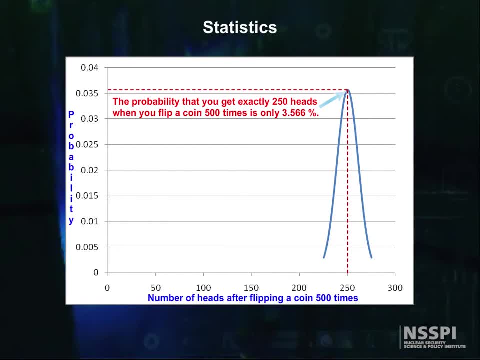 activity and radiation, and I'll show you some nifty things we can do with our decay constant.